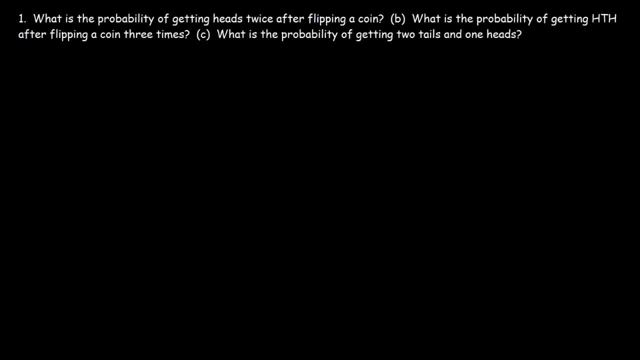 In this video we're going to focus on compound probability, but particularly of independent events. So let's say we wish to find a probability of two events occurring, Let's say event A and event B. If these events are independent, then the probability of these two events occurring 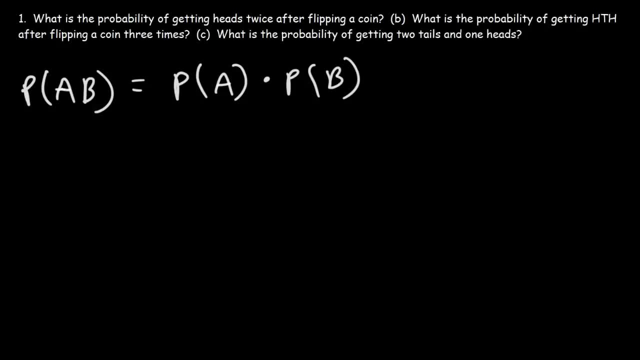 is simply the product of the probability that event A will occur and then event B will occur. So let's keep that in mind. Now let's focus on this question: What is the probability of getting heads twice after flipping a coin? So we need to get heads on the first try and then heads 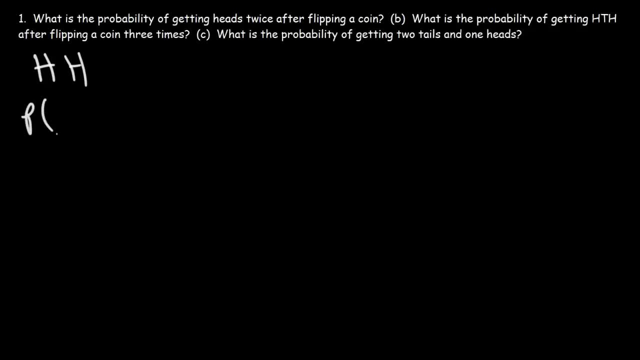 on the second try. So the probability of getting these two events is going to be: the probability of getting heads on the first try times the probability of getting heads on the second try. the probability of getting heads on a second try. So what is the probability of getting heads just by flipping one coin? 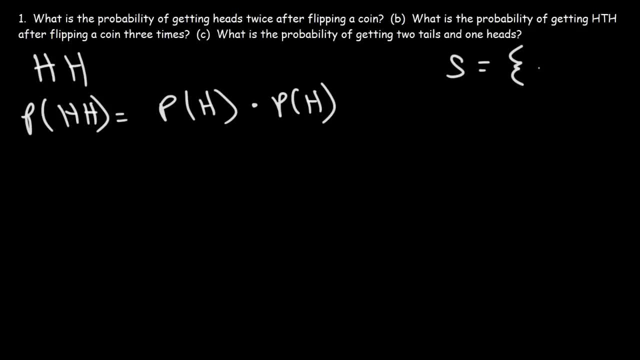 Well, if we write out the sample space, there's only two options. Either we get heads or tails. So the probability of getting heads is going to be this: one option out of the two possible options. So it's one out of two. 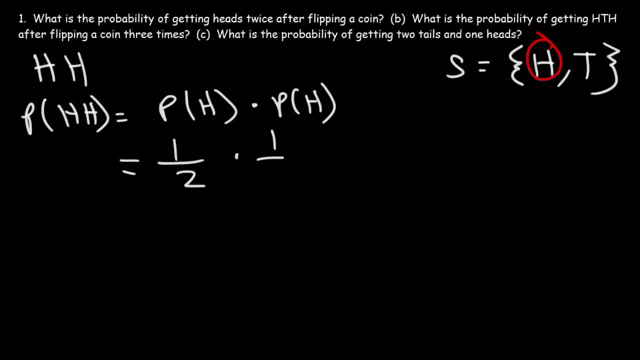 Now for the second event. the probability will be the same. It's also one out of two. One times one is one. two times two is four. So the probability of getting two heads is one out of four. Now to confirm this answer. 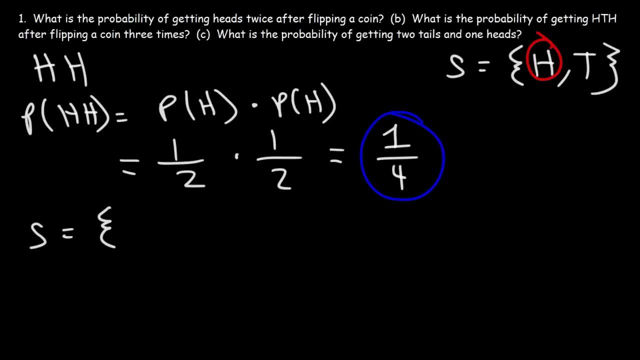 let's write out the sample space for flipping two coins. We can get heads and then heads, or we can get heads then tails, or we can get tails first and then heads on the second try, or we can get two tails. So notice that we have one event, that is our desired event, out of a potential of four events. 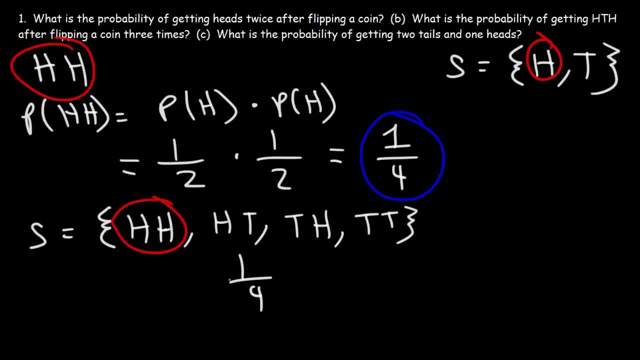 So that's why the probability is one out of four. Out of the four events, only one leads to a successful outcome- the outcome that we want- And so that's one way in which you can confirm that answer. Subtitles by the Amaraorg community. 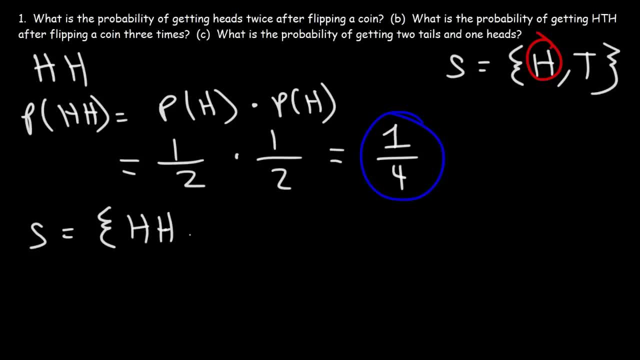 We can get heads and then heads, or we can get heads then tails, or we can get tails first and then heads on the second try, or we can get two tails. So notice that we have one event- that is our desired event, out of a potential of four events. So that's why 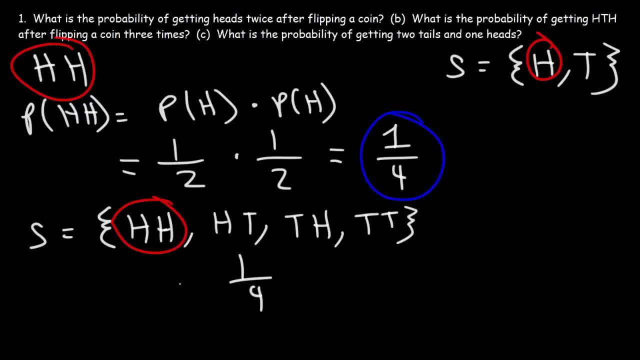 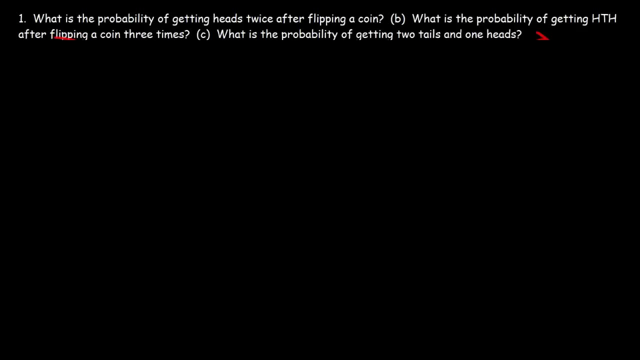 the probability is one out of four. Out of the four events, only one leads to a successful outcome, the outcome that we want, And so that's one way in which you can confirm that answer. Now, what about B? What is the probability of getting heads- tails- heads after flipping a coin three times? 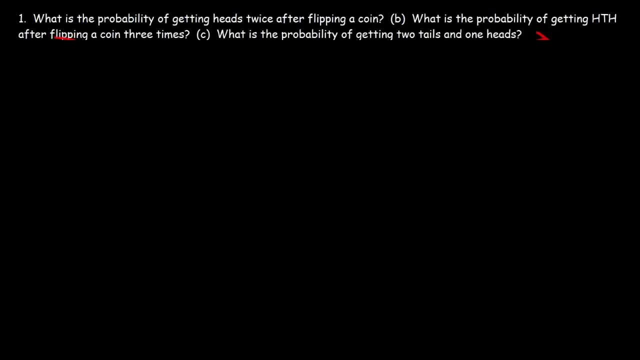 So what you need to know is that the order matters in this problem. But again, the answer is pretty straightforward. So, HTH, this is going to be the probability of getting heads on the first try times. the probability of getting tails on the second try times. the probability of getting heads. 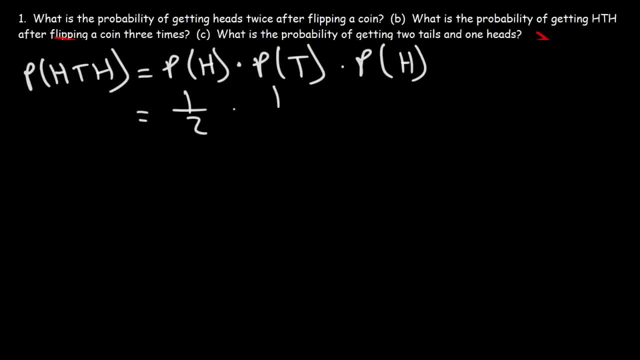 on the second try times the probability of getting tails on the second try, of getting heads on the the third try, and so for each of these events, the probability of them occurring is one half. so this is basically one half raised to the third power. two to the third is eight and one to the. 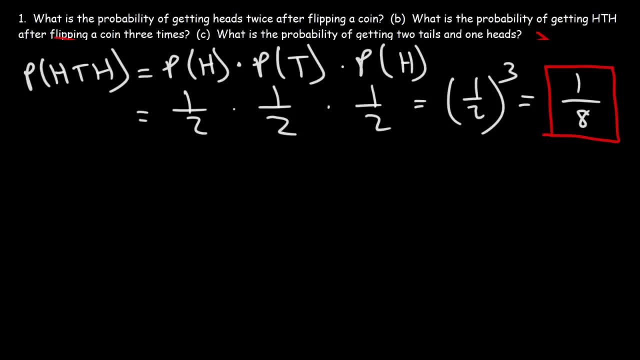 third is one, so the probability of this happening is one out of eight. now let's confirm it. let's write out the sample space for flipping three coins, so we can get all three heads. or it could be heads, heads and then tails, or it can be h, th or htt, thh, and so forth. so these are the. 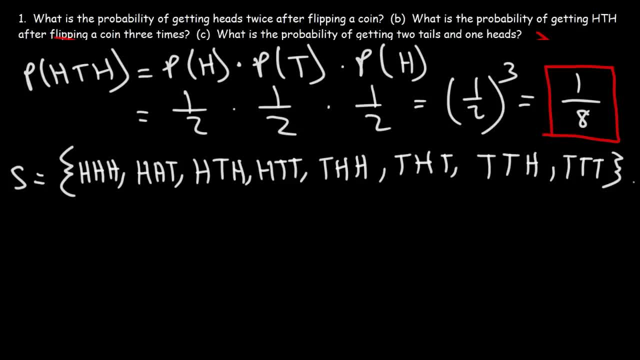 eight possibilities that we can get when flipping three coins. so notice that there's only one out of these eight possibilities that leads to the event that we want, and so that's why the probability is one out of eight. now let's move on to part c. what is the probability of? 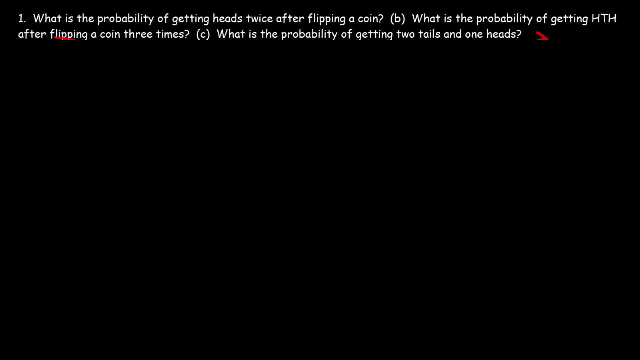 Now what about part b? What is the probability of getting heads, tails, heads after flipping a coin three times? So what you need to know is that the order matters in this problem, But getting the answer is pretty straightforward, So hth. 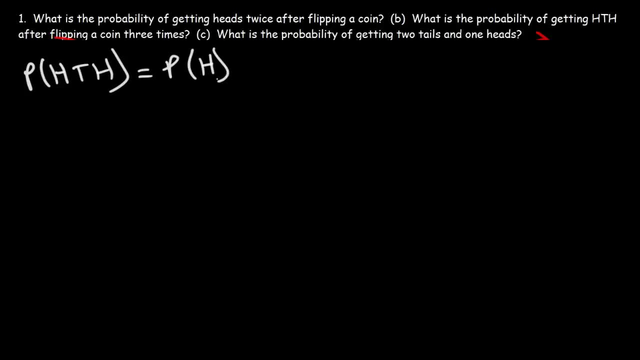 this is going to be the probability of getting heads on the first try times the probability of getting tails on the second try times the probability of getting heads on the third try, And so, for each of these events, the probability of them occurring is one half. 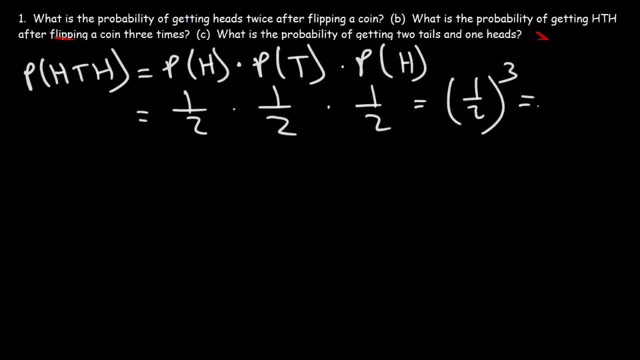 So this is basically one half raised to the third power. Two to the third is eight and one to the third is one. So the probability of this happening is one out of eight. Now let's confirm it. Let's write out the sample space for flipping three coins. 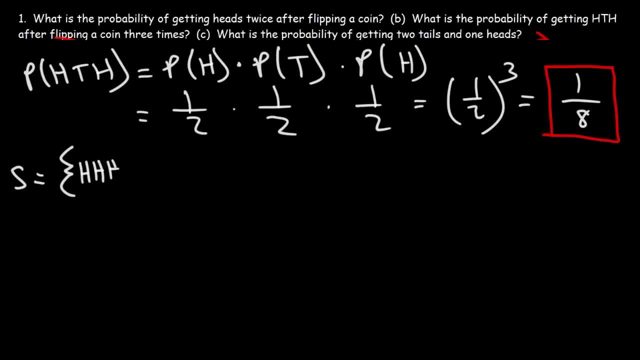 So we can get all three heads, or it could be heads, heads and then tails, or it can be H T H or H T T, T, H, H, and so forth. So these are the eight possibilities. 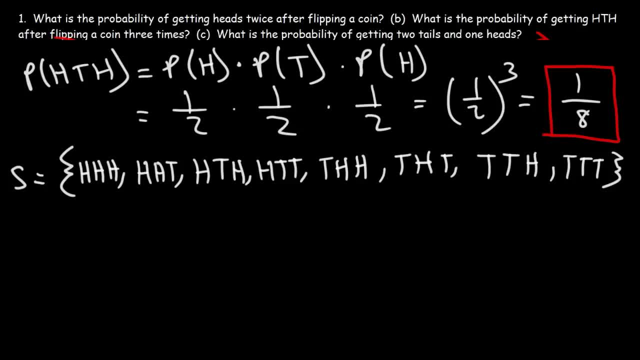 that we can get when flipping three coins. So notice that there's only one out of eight. There's only one out of these eight possibilities that leads to the event that we want, And so that's why the probability is one out of eight. 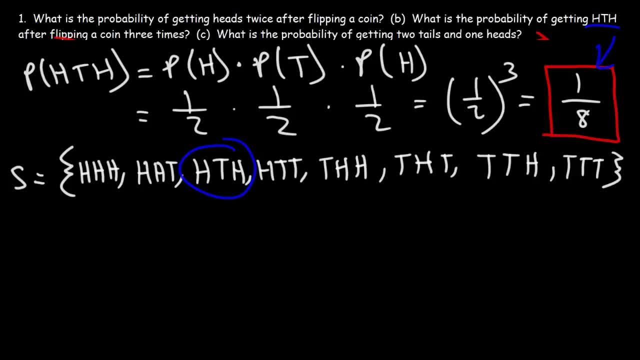 Now let's move on to part C. What is the probability of getting two tails and one heads? So does the order matter in this problem? So, looking at the eight options that we have here, which one contains two tails and one heads? I'm going to highlight it in red. 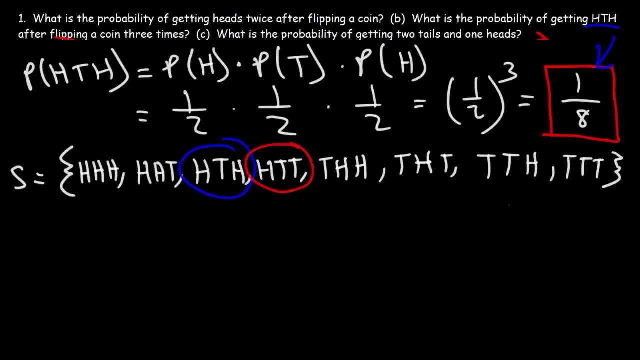 So this has two tails and one heads, So there's this one and that one as well. So therefore, the probability of getting either H T T or T H T or T T H is three out of eight. 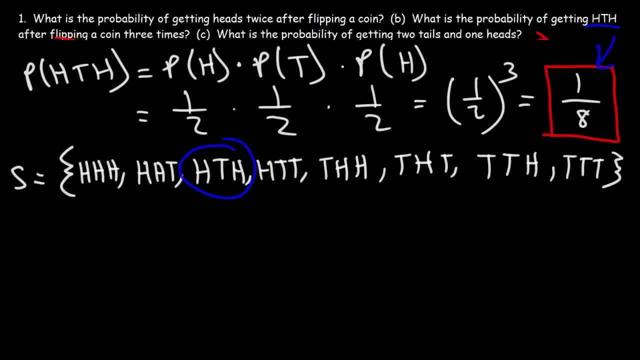 getting two tails and one heads. so does the order matter in this problem? so, looking at the eight options that we have here, which one contains two tails and one heads? i'm gonna highlight it in red. so this has two tails and one heads. so there's this one and that one as well. so therefore the probability. 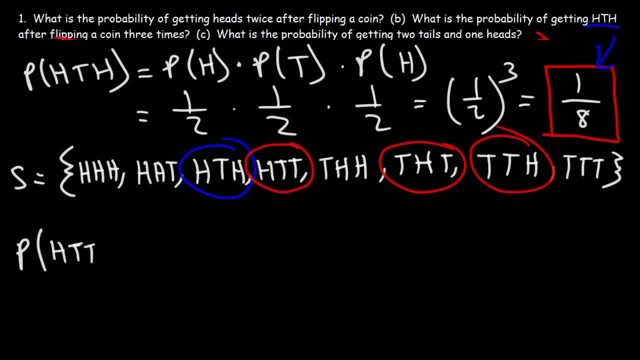 of getting either h t t or t h t or t t h is three out of eight, because we have three favorable outcomes out of eight possibilities that will lead to this event. so you need to be careful where you're looking at the order. is that the order is not going to matter, if the order matters or if it? 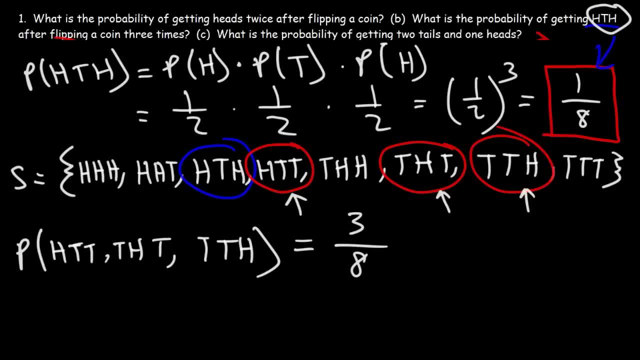 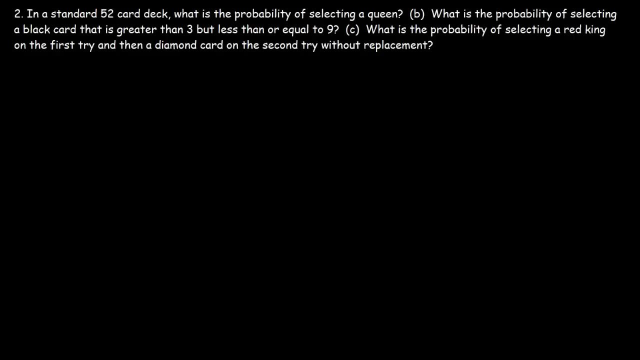 doesn't. so for this problem the order matters, but for the second problem the order doesn't matter. so it's good to list out all the potential events that would lead to this particular situation. number two: in a standard 52 card deck, what is the probability of selecting a queen? 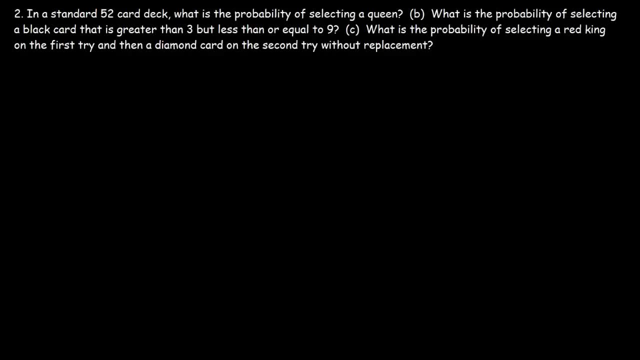 well, before we go into this question, let's talk about some things you need to know. so in a standard 52 card deck you don't have any jokers. the first type of card that you have is the red diamond. the second card is the red hearts, the third one, which is going to be black- but i can't use black on. 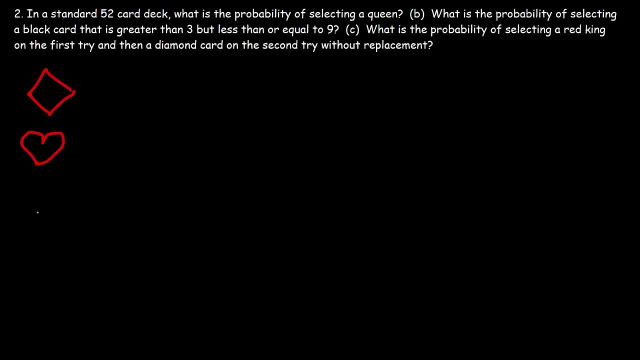 a black screen, so i'm going to use white instead. the third one represents the spades, which looks something like this: my drawing's not perfect, but what you can do is go to google images, type in standard 52 card deck and you'll see all the cards in the 52 card deck. 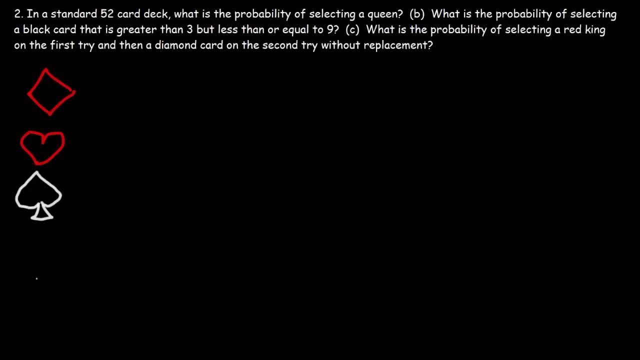 but this is supposed to be black instead of white. just keep that in mind. the last type is the clubs, which looks something like this: let me see if i can draw that better, but it's something like that. you'll see it when you uh search on google images. now for each of these four different types of cards. 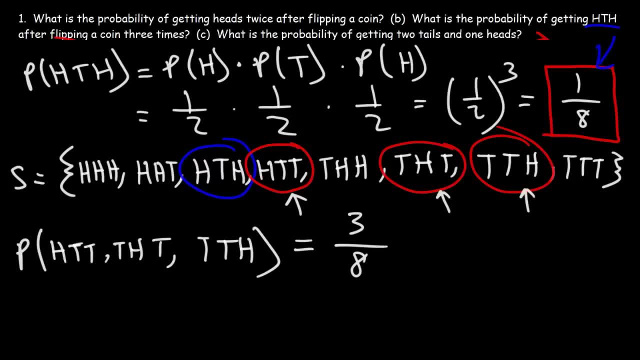 because we have three favorable outcomes out of eight possibilities That will lead to this event. So you need to be careful where: if the order matters or if it doesn't. So for this problem the order matters, but for the second problem, the order doesn't matter. 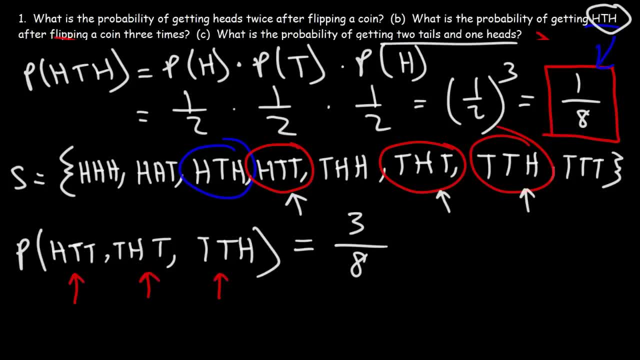 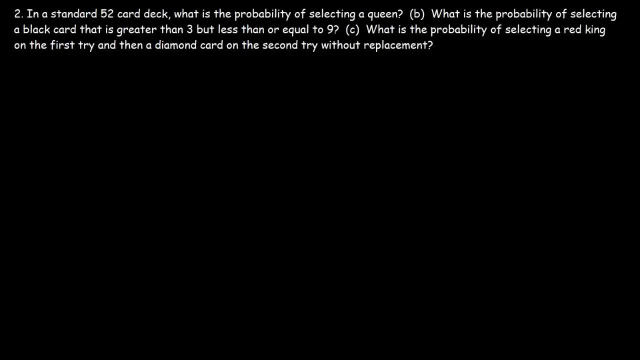 So it's good to list out all the potential events that would lead to this particular situation. Number two: in a standard 52 card deck, what is the probability of selecting a queen? Well, before we go into this question, I'm going to go into this question. 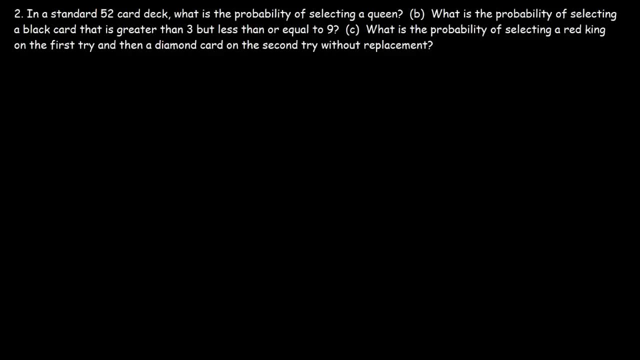 Let's talk about some things you need to know. So in a standard 52 card deck you don't have any jokers. The first type of card that you have is the red diamond. The second card is the red hearts, The third one, which is going to be black, 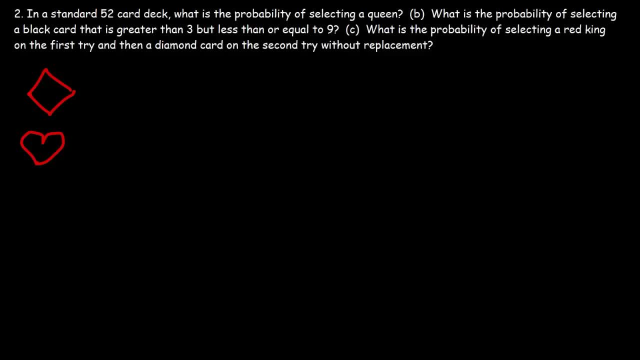 but I can't use black on a black screen, So I'm going to use the white instead. The third one represents the spades, which looks something like this: My drawing's not perfect, but what you can do is go to Google Images. 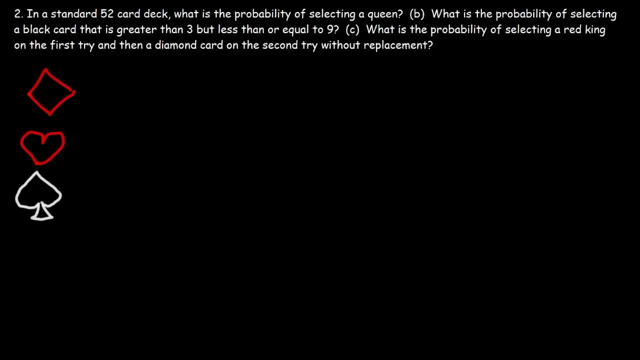 type in standard 52 card deck and you'll see all the cards in the 52 card deck. But this is supposed to be black instead of white. Just keep that in mind. The last type is the clubs, which looks something like this: 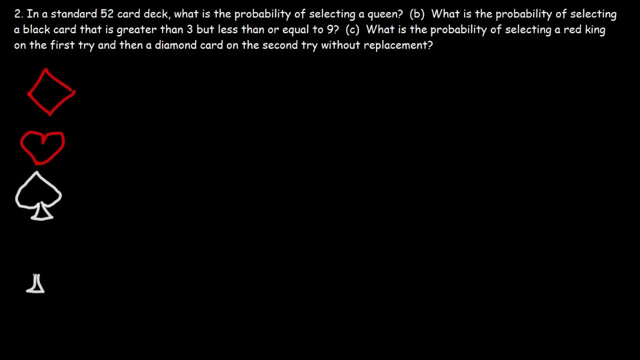 Let me see if I can draw that better, But it's something like that. You'll see it when you search it on Google Images. Now, for each of these four different types of cards, you have the ace and then you have the numbers two. 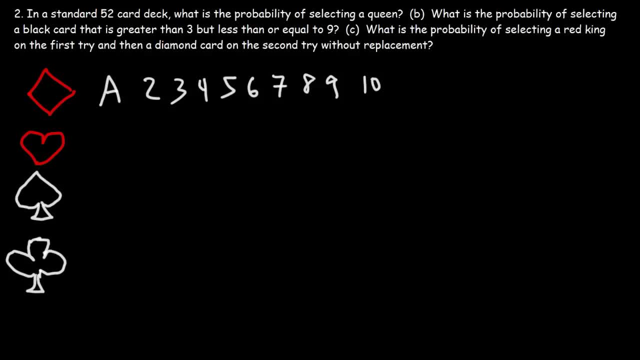 all the way to 10.. After 10, you have the jack and then the queen and then the king. So this right here represents 13 cards. So what this means is that there's 13 diamonds, 13 hearts. 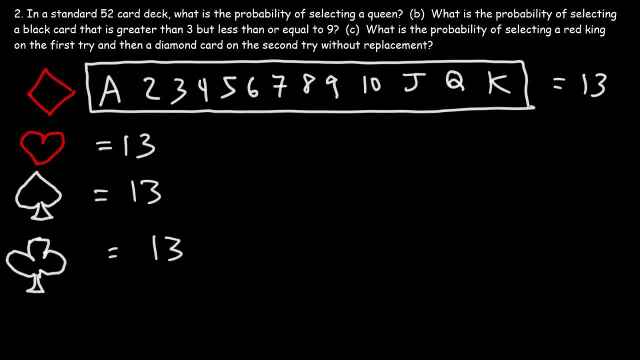 13 spades and 13 clubs. 13 times four gives us the total of 52 cards. So there's two types of cards that are red. 13 times two is 26.. So there's 26 red cards and there's 26 black cards. 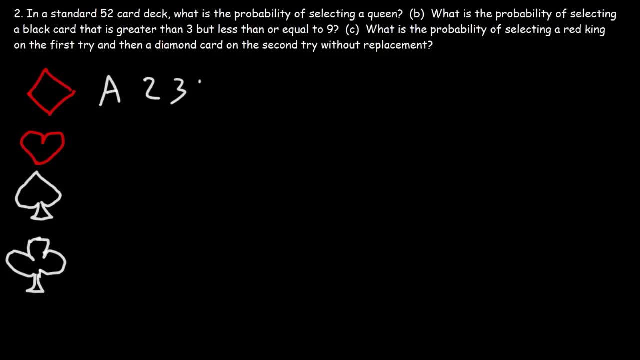 you have the ace and then you have the numbers two, all the way to ten. after ten you have the jack and then the queen and then the king. so this right here represents 13 cards. so what this means is that there's 13 diamonds, 13 hearts. 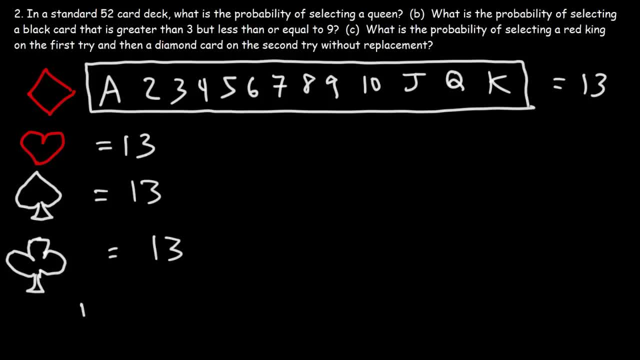 13 spades and 13 clubs. 13 times 4 gives us the total of 52 cards. so there's two types of cards that are red. 13 times 2 is 26.. so there's 26 red cards and there's 26 black cards. 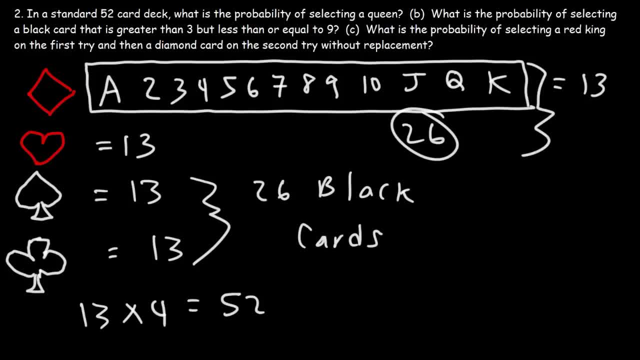 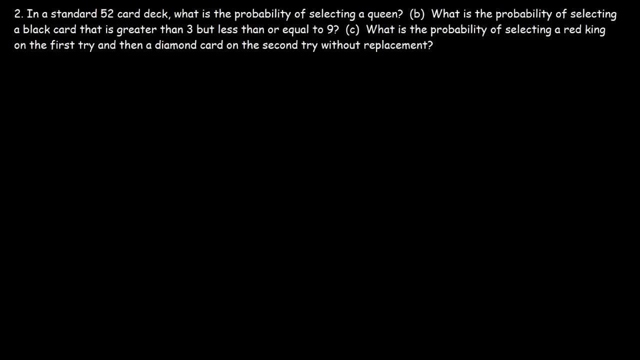 so these are some things to know if you're dealing with a probability question using cards, so let's begin. you may want to write those things down as notes to answer these questions coming up. so, in a standard 52 card deck, what is the probability of selecting a queen? 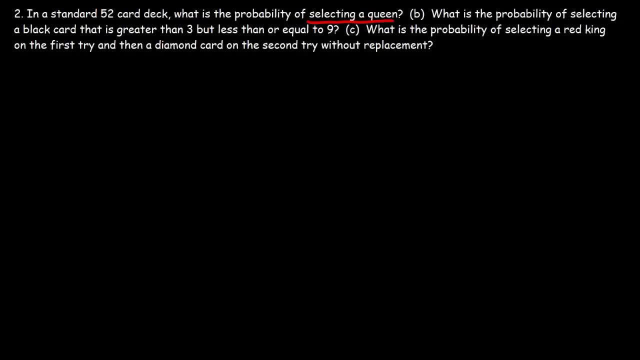 so how many queens are there? so we have the queen of diamonds, the queen of hearts, the queen of spades and the queen of clubs. so there's only four types of queens because there's four different types of cards. so there's four queens out of a total of 52 cards. 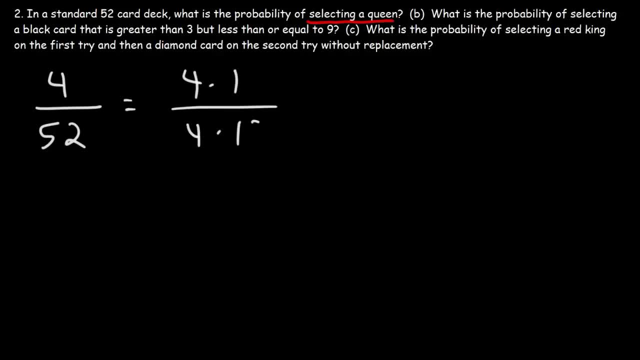 4 is 4 times 1, 52 is 4 times 13.. so we could cancel a 4, and so the answer is going to be 1 out of 13.. 1 divided by 13 is basically 0.07692. that's a rounded answer. so if you multiply that by 100, 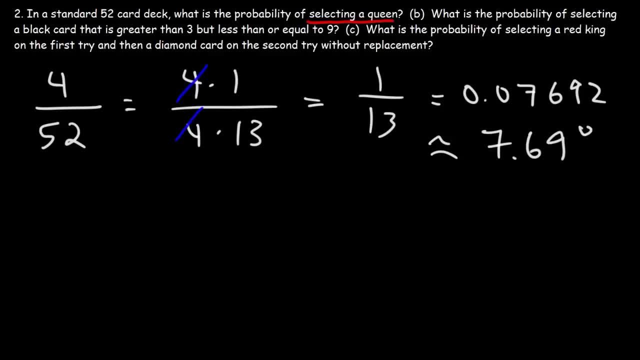 the probability is approximately 7.69. now what about part b? what is the probability of selecting a black card that is greater than 3 but less than or equal to 9.. so let's write out the list of numbers that fit these characteristics. so let's say that x is basically the number of a card that we're going to pick. 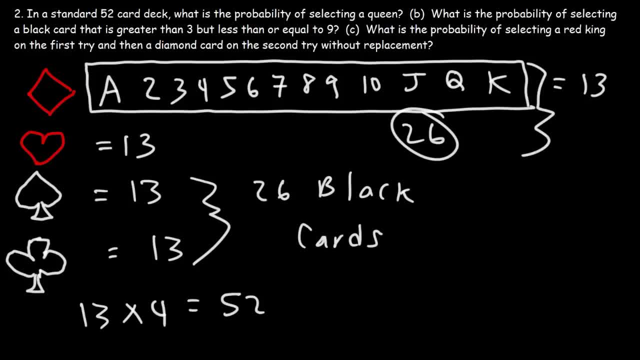 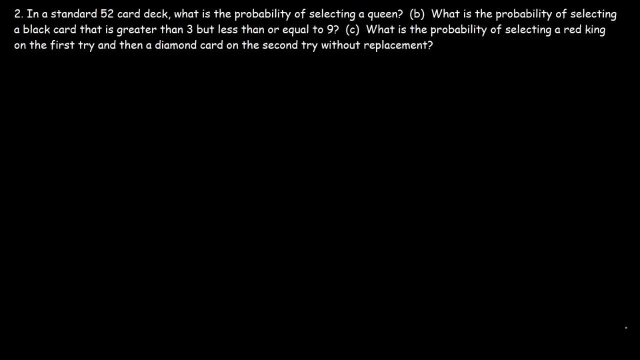 So these are some things to note. Here's the know. if you're dealing with a probability question using cards, So let's begin. You may want to write those things down as notes to answer these questions coming up. So in a standard 52 card deck. 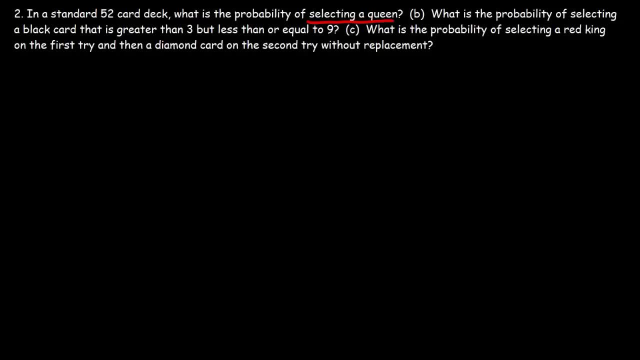 what is the probability of selecting a queen? So how many queens are there? So we have the queen of diamonds, the queen of hearts, the queen of spades and the queen of clubs. So there's only four types of queens, because there's four different types of cards. So there's four queens out of a. 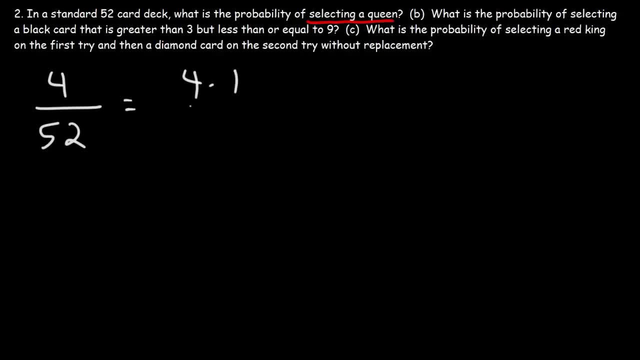 total of 52 cards. Four is four times one. Fifty-two is four times thirteen, So we could cancel a four, and so the answer is going to be one out of thirteen. One divided by thirteen is basically point zero. Seven, six, nine, two. That's a rounded answer. So if you multiply that by a hundred, 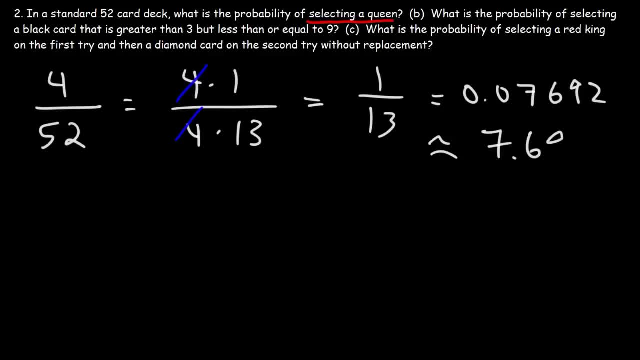 the probability is approximately seven point six nine percent. Now what about part B? What is the probability of selecting a black card that is greater than three but less than or equal to nine? So let's write out the list of numbers that fit these characters. 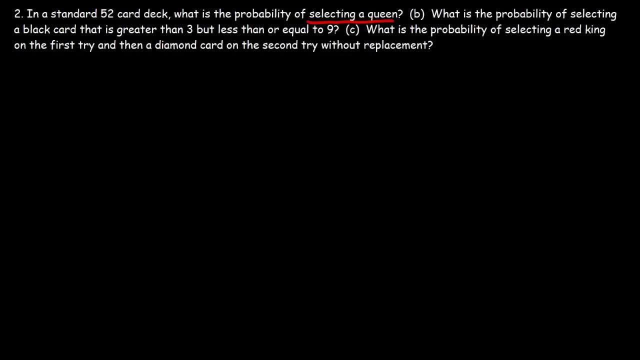 So let's say that X is basically the number of a card that we're going to pick. It's greater than three, but less than or equal to nine. So this does not include three. So if we write the sample space, this is going to be four, five, six, seven, eight, nine. Now you might be thinking: 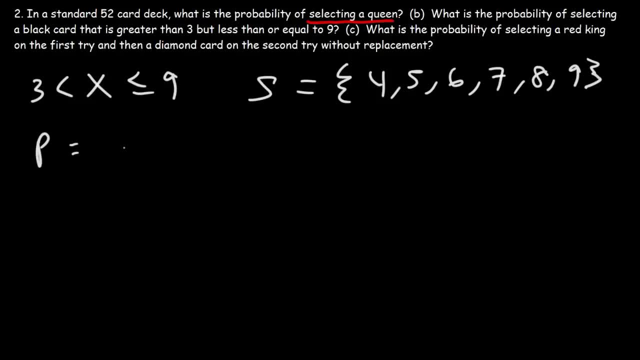 okay, so the probability is going to be six out of fifty-two. But keep in mind there's two types of black cards. You have the clubs and you have the spades. So there's six black clubs with these numbers and there's six spades with those same numbers. So really there's twelve cards, that is. 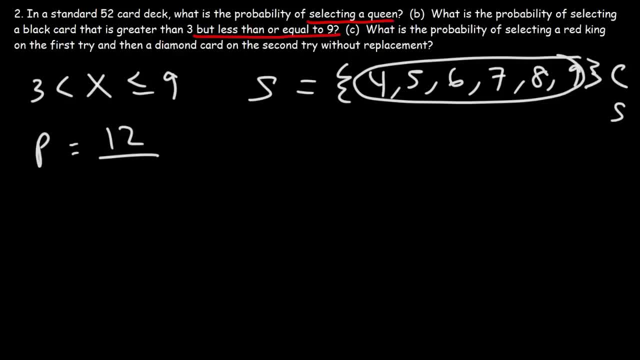 between that's greater than three, less than or equal to nine, That is a black card Because you got the clubs and the spades. So it's twelve out of fifty-two. Twelve is four times three. Fifty-two is four times thirteen. So if we cancel a four, the probability 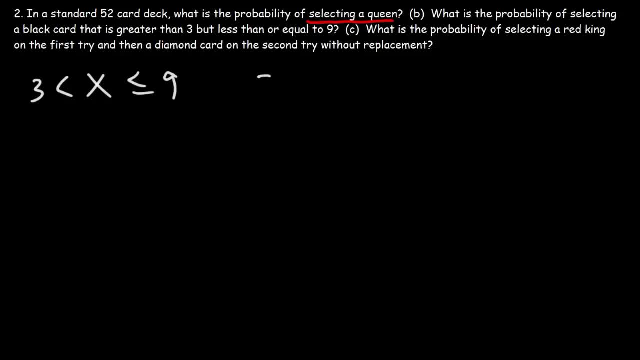 it's greater than 3, but less than or equal to 9.. so this does not include 3.. so if we write the sample space, this is going to be 4, 5, 6, 7, 8, 9.. now you might be thinking: 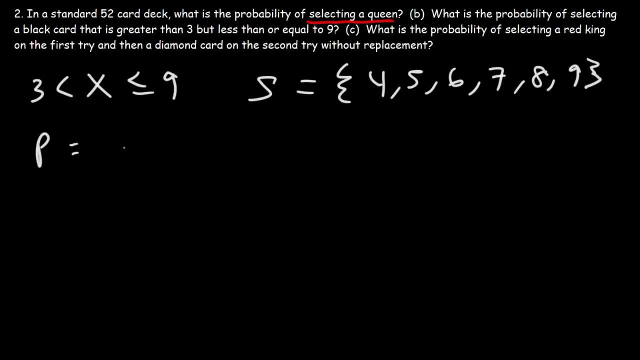 okay, so the probability is going to be 6 out of 52. but keep in mind there's two types of black cards. you have the clubs and you have the spades. so there's six black clubs with these numbers and there's six spades with those same numbers. so really there's 12. 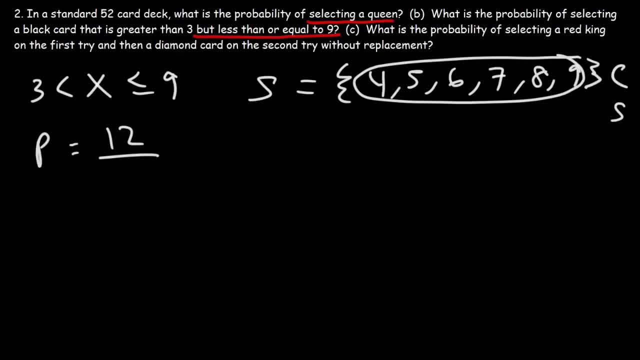 cards. that is between that's greater than 3, less than or equal to 9. that is a black card, because you got the clubs and the spades. so it's 12 out of 52.. 12 is 4 times 3. 52 is 4 times 13.. 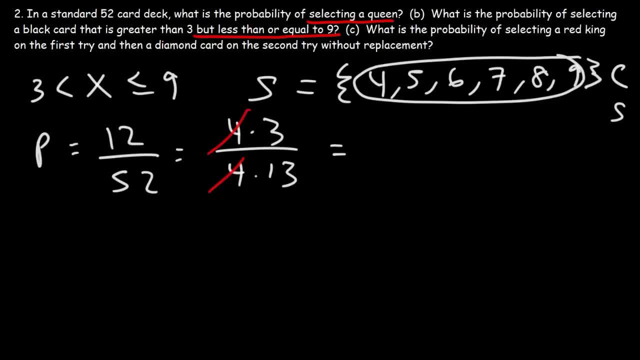 so if we cancel a 4. the probability is going to be three out of 13.. This is the answer for part B. Now let's move on to our last question, or rather the last part in this question, Part C: what is the probability? 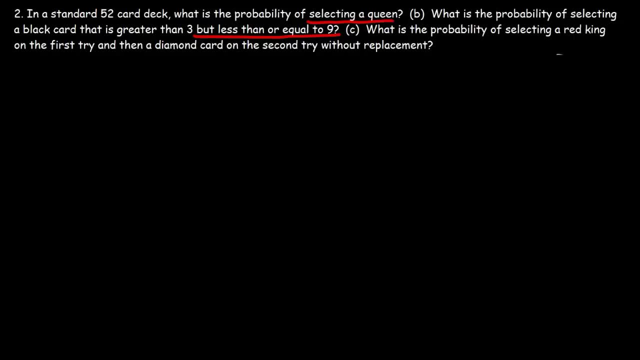 of selecting a red queen on not a red queen, but a red king on the first try, and then a diamond card on the second try, without replacement. Now, this problem is a little bit tricky, so go ahead and try it Now. what we don't want to do is this: We don't want to say 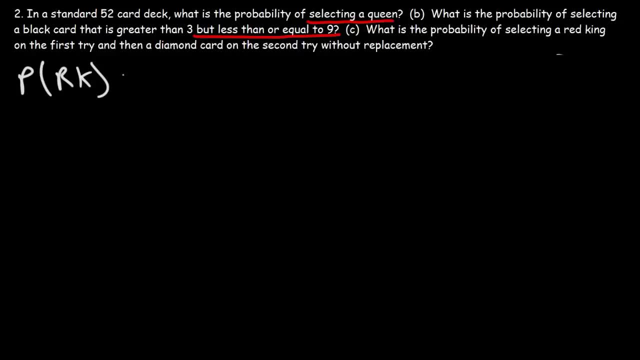 it's going to be the probability of selecting a red king times the probability of selecting a diamond, because the first event is going to affect the second event. For instance, let's say, if we want to find the probability of selecting a red king, There's two red kings out. 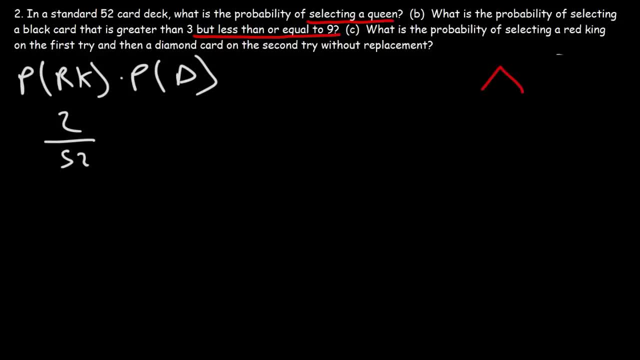 of 52 cards. You could have the red diamond or the red king of hearts. Now the probability of selecting a diamond without replacement. we took out a card, so there's 51 cards left. Now how many diamonds are left Now? the number of diamonds that are left depends on: 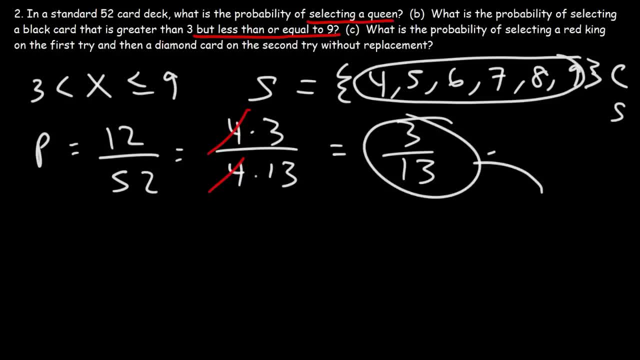 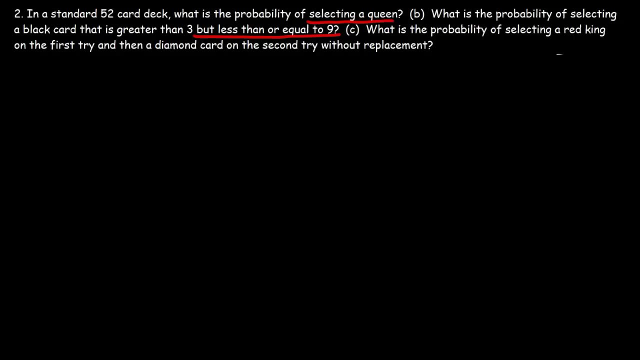 is going to be three out of thirteen. This is the answer for part B. Now let's move on to our last question, or rather the last part in this question, Part C: what is the probability of selecting a red queen on not a red queen, but a red king on the first try? 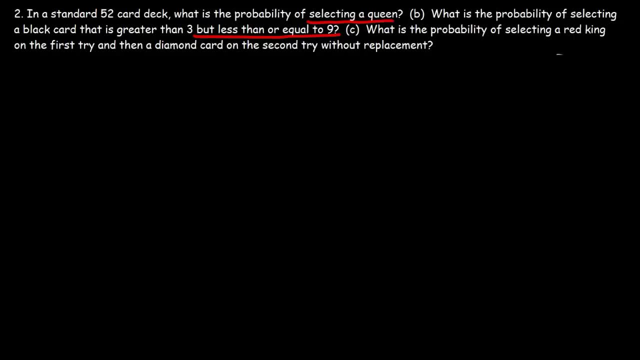 And then a diamond card on the second try, without replacement. Now this problem is a little bit tricky, So go ahead and try it Now. what we don't want to do is this. We don't want to say it's going to be the probability of selecting a red king times the probability of selecting a diamond. 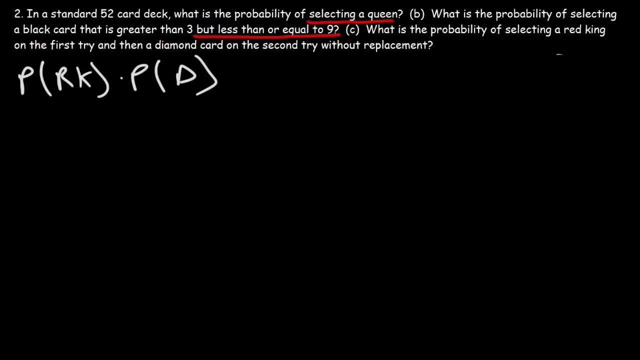 Because the first event is going to affect the second event. For instance, let's say, if we want to find the probability of selecting a red king, there's two red kings out of fifty-two cards. You could have the red diamond or the red king. 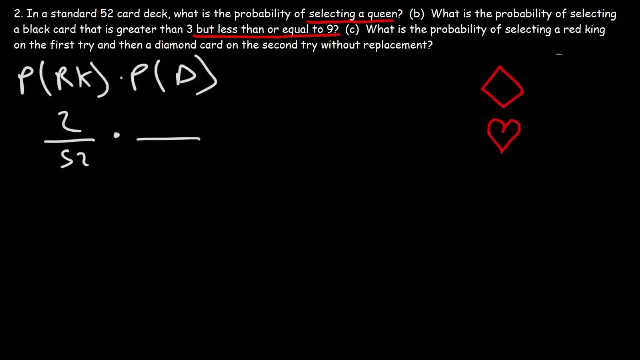 of hearts. Now the probability of selecting a diamond without replacement. we took out a card, so there's fifty-one cards left. Now how many diamonds are left? Now, the number of diamonds that are left depends on which red king that you selected. If we selected a red king of 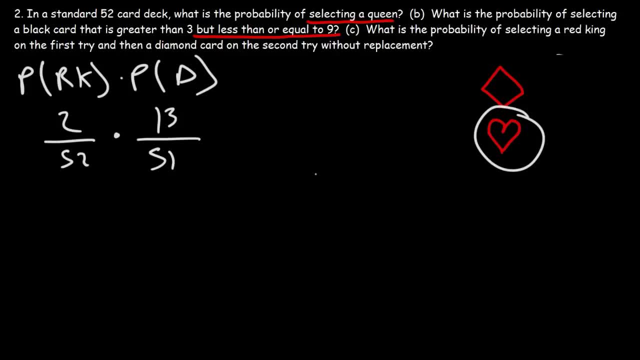 hearts, then there's thirteen diamonds left, including the red king of diamonds. But if on the first try we selected the red king of diamonds, then there's twelve diamonds left. So these are dependent events. The second event depends on the first event, so we can't 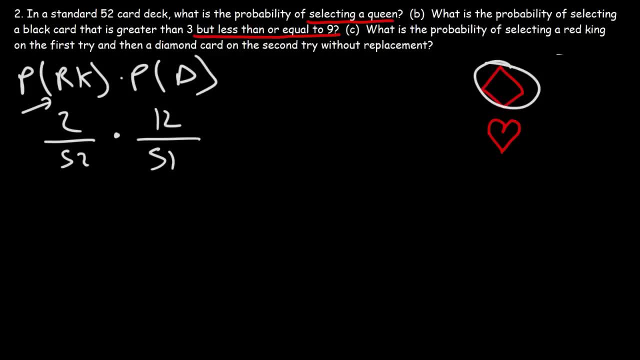 use this equation for this particular situation. Now, another formula that we could use is: when you have an or situation, The probability of selecting A or B is equal to the probability of A plus the probability of B. We're going to have to use this, So event A is going to represent the first situation, That is, let's 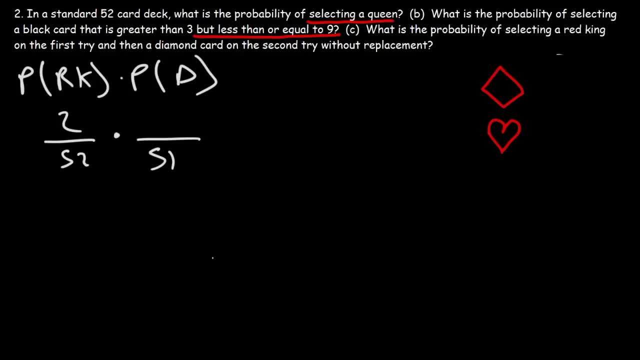 which of the red kings are left. So we're going to take out a red king and we're going to take out which red king that you selected. If we selected a red king of hearts, then there's 13 diamonds left, including the red king of diamonds. But if, on the first try, we selected 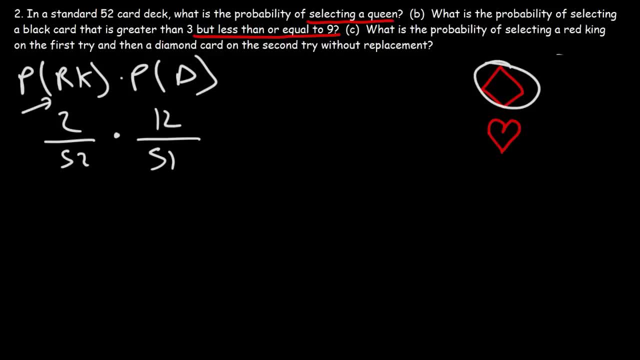 the red king of diamonds, then there's 12 diamonds left. So these are dependent events. The second event depends on the first event, so we can't use this equation for this particular situation. Now, another formula that we could use is: when you have an or situation, The probability. 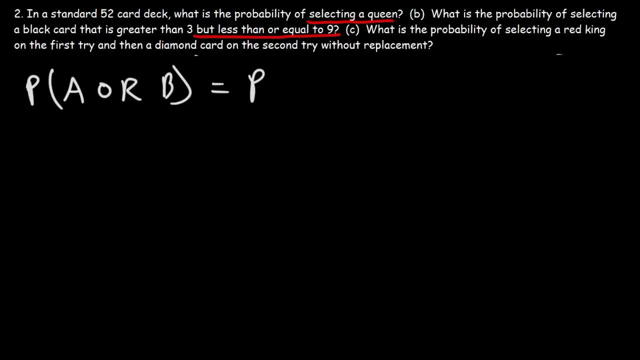 of selecting A or B is equal to the probability of A plus the probability of B. We're going to have to use this, So event A is going to represent the first situation, That is, let's say, if we select a red king of hearts. 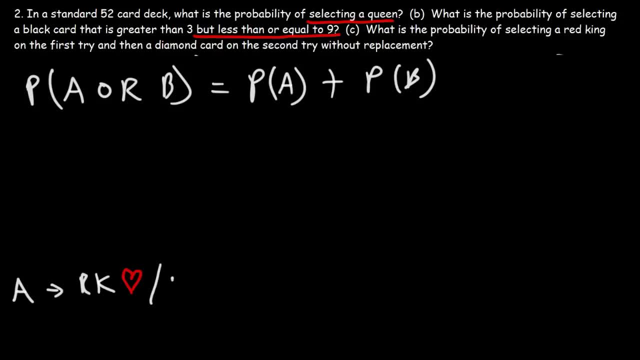 And then, on the second event, we'll be selecting a diamond. Event B will be selecting a red king of diamonds, And then the second event will be selecting another diamond card. So let's start with the first event. This is going to be the probability of getting. 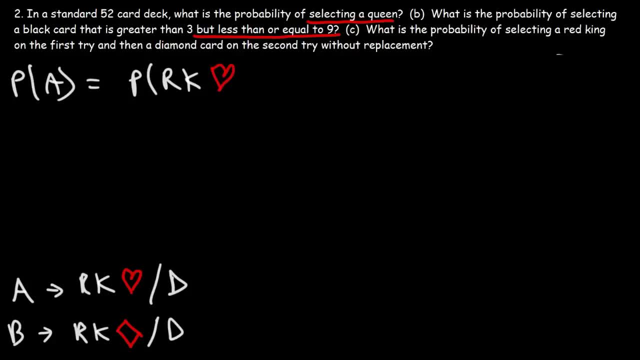 the red king of hearts, And then the third event is going to be the probability of getting the red king of hearts. So we know that there's four red kings. I mean, there's four king cards. Two of them are red: The diamonds and the hearts. So to get a red king of hearts there's only one. 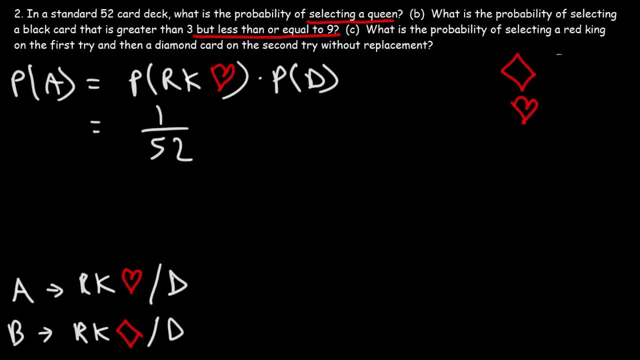 red king of hearts out of 52 cards. So the probability is one out of 52.. Now to get a diamond card. after that, we're going to have to do the following: We're going to take out the red king. Once we take out the red king, there's going to be not 52 cards. 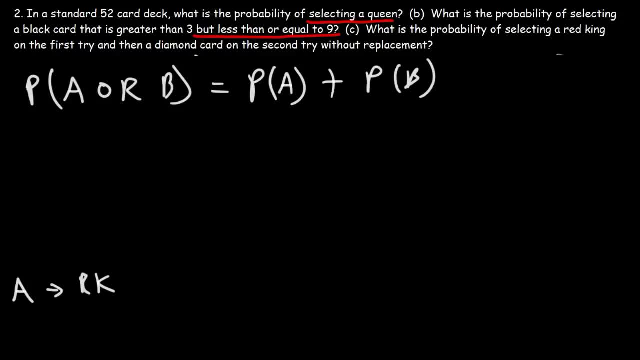 say, if we select a red king of hearts And then on the second event we'll be selecting a diamond, Event B will be selecting a red king of diamonds And then the second event will be selecting another diamond card. So let's start with the first event. This is going to be the probability of getting. 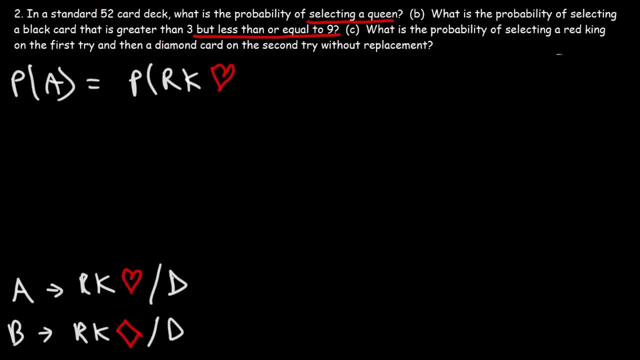 the red king of hearts Times the probability of getting a diamond card. So we know that there's four red kings. I mean there's four king cards. Two of them are red: the diamonds and the hearts. So to get a red king of hearts, there's only one red king of hearts out of 52 cards. So the 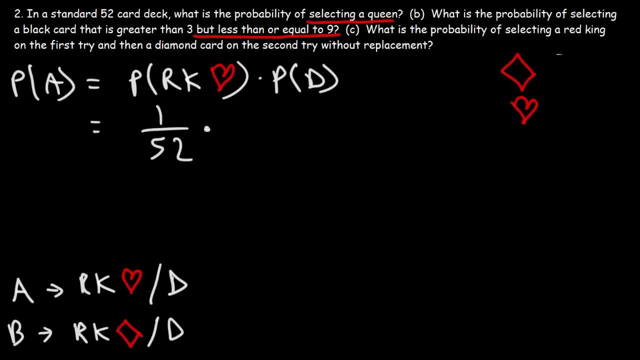 probability is one out of 52.. Now to get a diamond card. after that there's once we take out the red king, there's going to be not 52 cards in the deck, 51 cards, because this is without replacement. We're not putting. 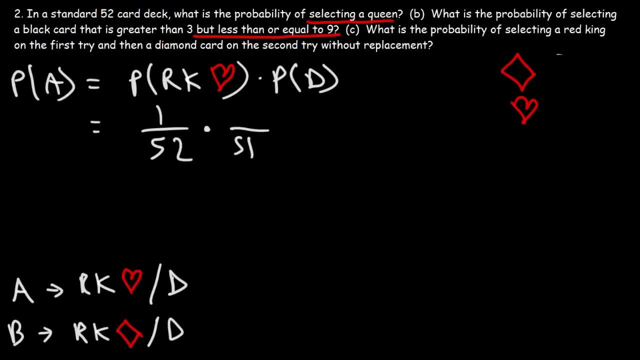 the red king of hearts back into the deck. So now we have 51 cards to choose from. 13 of those cards are diamonds. So now let's do the math. 52 is basically four times 13.. So we can cancel a 13.. And four times 50 is 200. So four times 51 is going to be 204.. You just add another four. 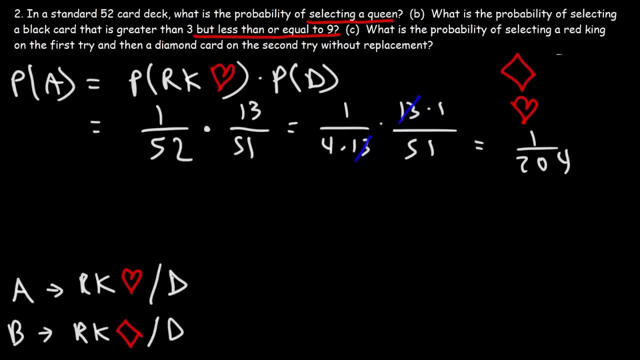 So the probability of getting a red king of hearts and then a diamond card is one out of 204.. Now let's focus on the other events. event B: So this is: if we get a red king of diamonds. When we put the probability of getting a red king of diamonds times, the 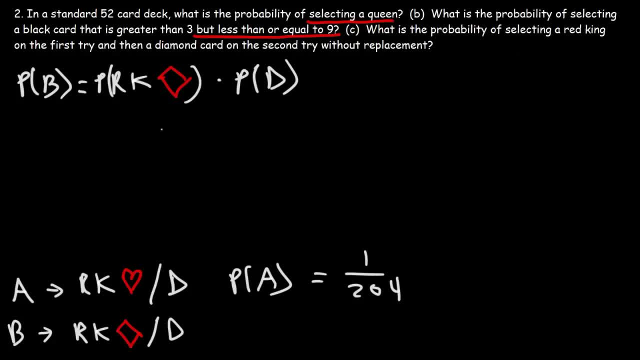 probability of getting a diamond card. There's only one red king of diamonds out of the 52 cards. Now, this is without replacement. Once we take that card out, there's one cards left. Now there's 13 diamond cards. we took out one of the diamond cards, so that's. 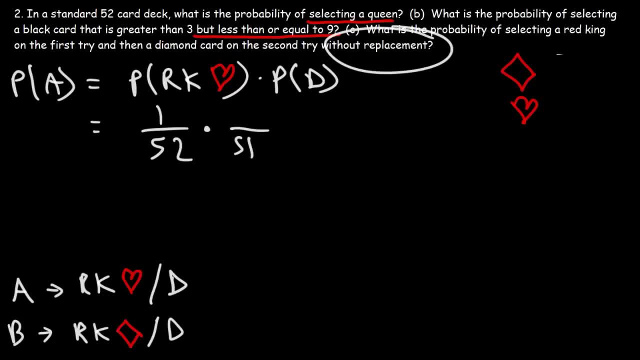 in the deck- 51 cards, because this is without replacement. We're not putting the red king of hearts back into the deck. So now we have 51 cards to choose from. 13 of those cards are diamonds. So now let's do the math. 52 is basically four times 13.. So we can cancel. 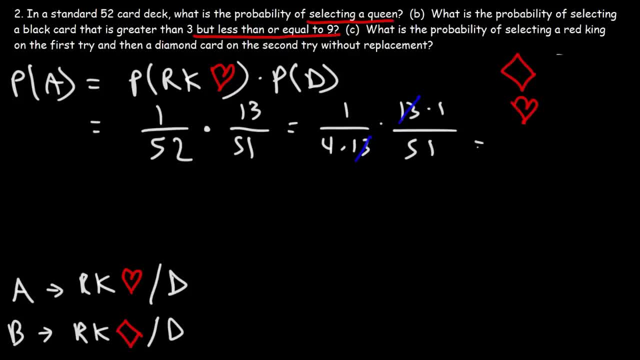 a 13.. And 4 times 50 is 200. So 4 times 51 is going to be 204.. You just add another 4.. So the probability of getting a red king of hearts and then a diamond card is one out. 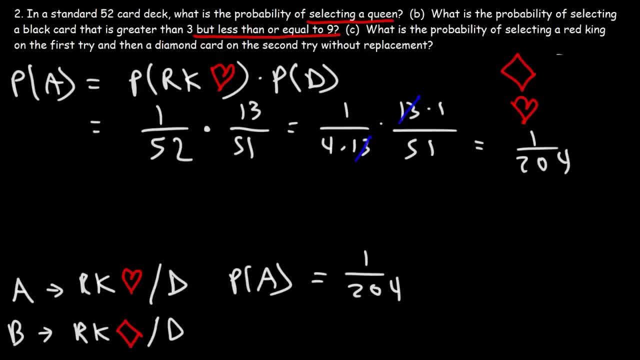 of 204.. Now let's focus on the other events. Event B: So this is: if we get a red king of diamonds. Let me put the probability of getting a red king of diamonds times the probability of getting a diamond card, So there's only one. 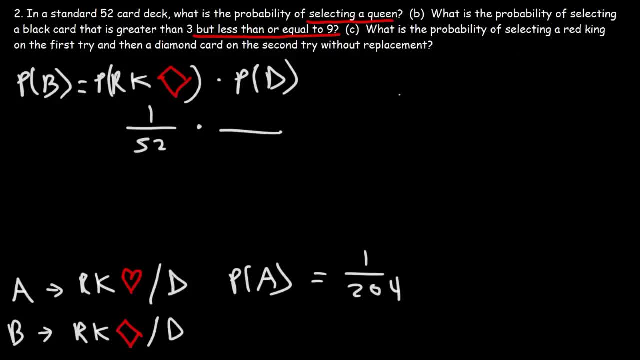 red king of diamonds out of the 52 cards. Now this is without replacement. Once we take that card out, there's 51 cards left. Now there's 13 diamond cards. We took out one of the diamond cards, So that's. 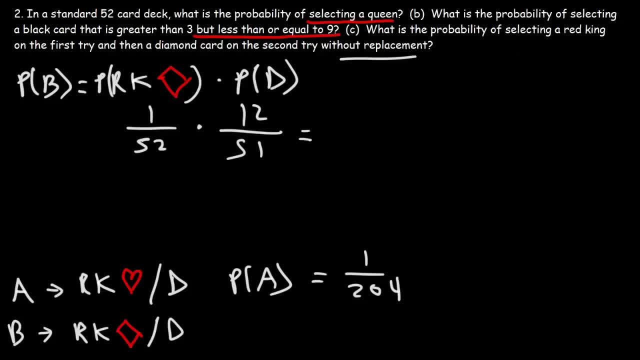 That's the number of cards left over. So the probability for the second event is going to be the 12 diamonds out of the 51 cards that remains 52, we're going to say it's 4 times 13.. 12 is 4 times 3.. 51 is 17 times 3.. So we're going to cancel a 4 and we're. 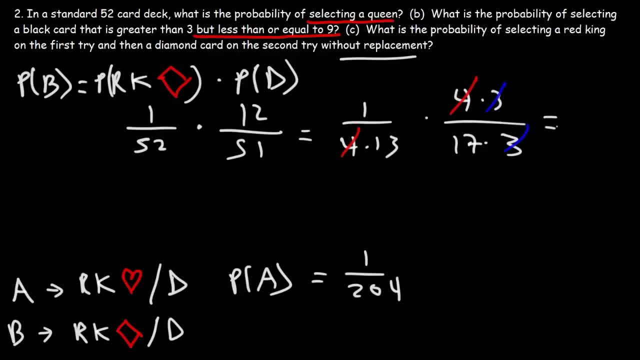 going to cancel a 3.. So what we have on the bottom is 13 times 17.. 13 times 17 is 4.. 4 times 17 is 221.. So the probability of selecting a red king of diamonds on the first try and then a diamond. 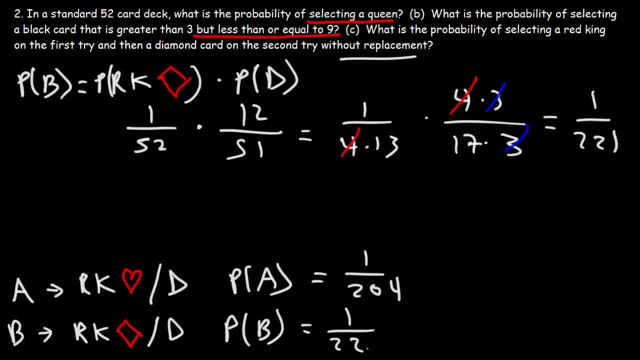 card on the second try, without replacement, is 1 out of 221.. Now let's put all of this together. So the probability of getting a red king followed by a diamond card- 1 out of 221- is the sum of the probability of getting a red king of hearts, because that 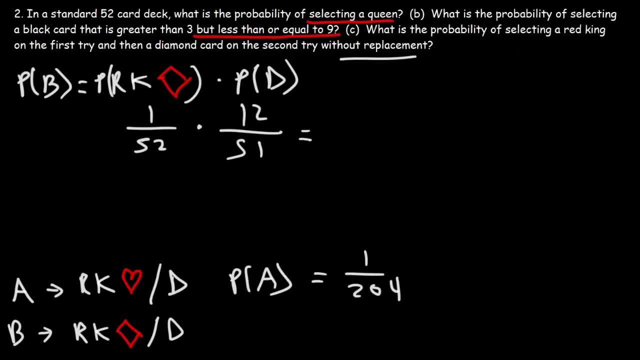 there's 12 diamond cards left over. So the probability for the second event is going to be the 12 diamonds out of the 51 cards that remains 52, we're going to say it's 4 times 13.. 12 is 4 times 3.. 51 is 17 times 3.. So we're going to cancel a 4 and we're going to cancel a 3.. 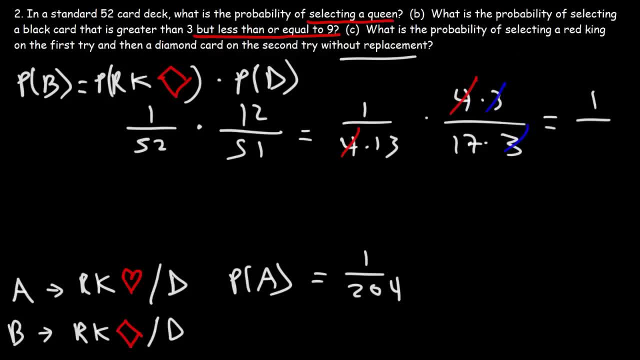 So what we have on the bottom is 13 times 17.. 13 times 17 is 221.. So the probability of selecting a red king of diamonds on the first try and then a diamond card on the second try, without replacement, is 1 out of 221.. Now let's put all of this together. 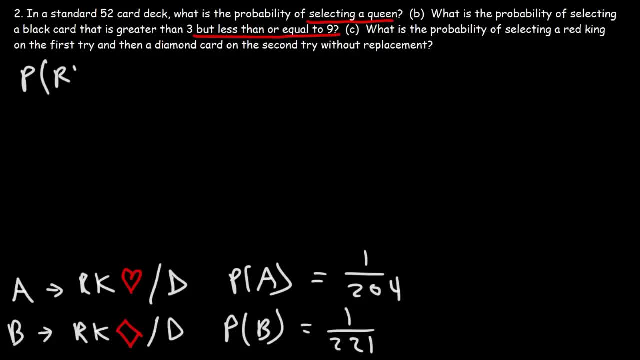 So the probability of getting a red king followed by a diamond card is the sum of the probability of getting a red king of hearts, because that is a red king, followed by a diamond card, plus the probability of getting a red king of diamonds, which is still a red king, followed by a diamond. 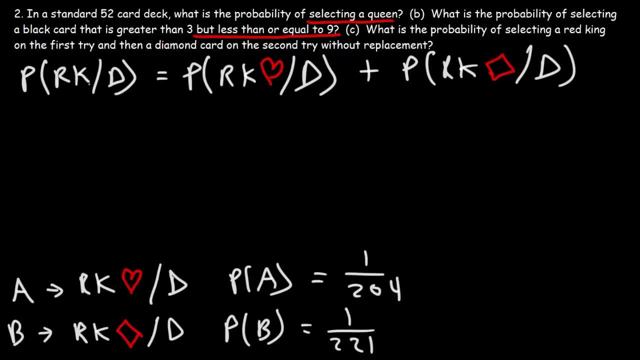 card. We have to break up this problem into these two. We have to break up this problem into these two situations because the probability for those two situations are different. So this is going to be 1 over 204 and then the other one is 1 over 221.. 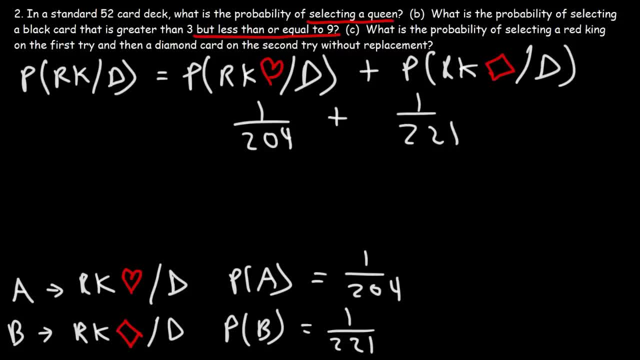 So we need to get common denominators in order to add these two fractions. Let's multiply the second fraction by 204 and the first one by 221.. 204 times 221 is 45,084, and then we can add 221 plus 204, which is 425.. 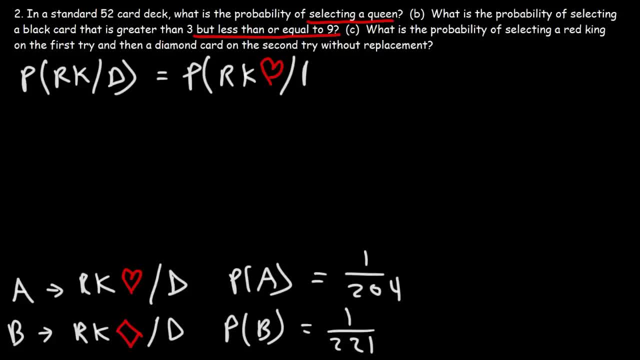 is a red king, followed by a diamond card, plus the probability of getting a red king of diamonds, which is still a red king, followed by a diamond card. We had to break up this problem into these two situations because the probability for those two situations are different. 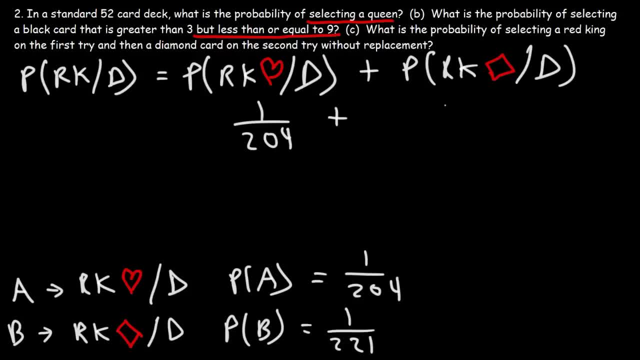 So this is going to be 1 over 204, and then the other one is 1 over 221.. So we need to get common denominators in order to add these two fractions. Let's multiply the second fraction by 204 and the first one by 221.. 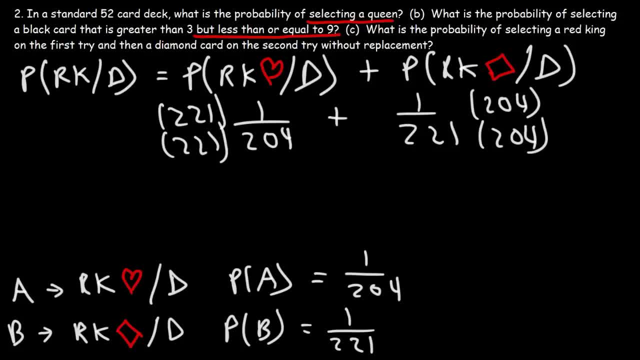 204 times 221 is 45,084.. And then we can add 221 plus 204.. So we have a red king of hearts, 204, which is 425.. Now we can probably simplify our answer somehow. These are some large numbers, so this is. 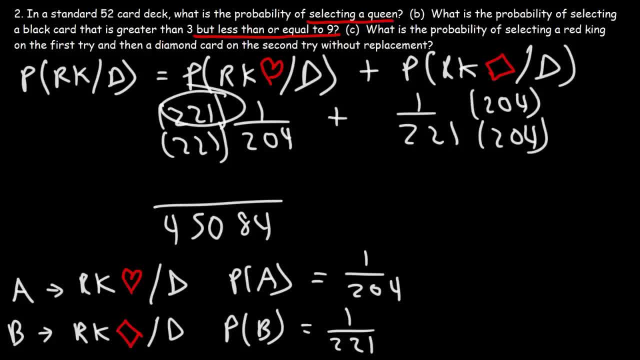 Let's take a step back. Perhaps it's better if we simplified it from the beginning. Now, 221, that's basically. we said that was 13 times 17.. 204 is 51 times 4.. Now 51, we can break that into 17 times 3.. 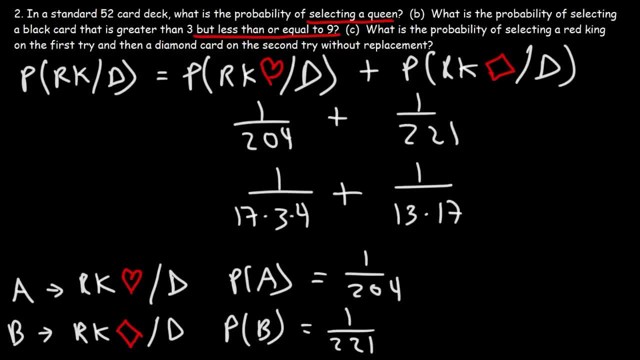 So 17 times 3 times 4, that'll give us the original 204.. So now we need to get common denominators. We already have a 17.. This has a 12, that's 3 times 4.. So we need to multiply the fraction on the right by 12 over 12.. 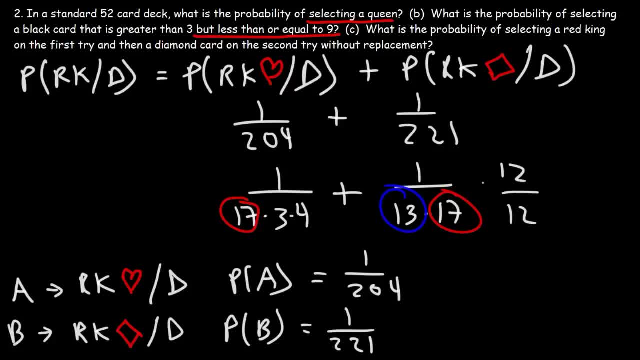 The fraction on the right has a 13, which the left one or the one on the left doesn't have. So we're going to multiply the fraction on the left by 13 over 13.. So this should give us commonator.